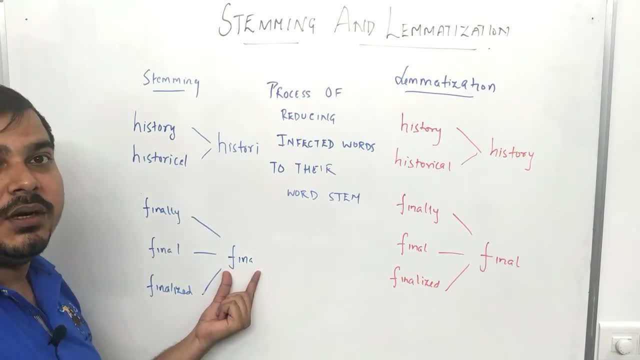 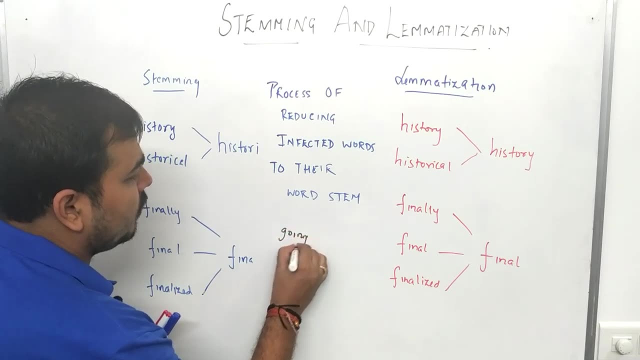 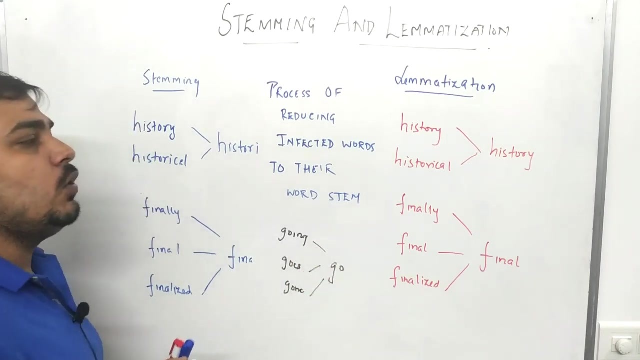 Right. So this is going to get reduced and we are actually getting this vertical word itself, fina. There are also some use cases like: if I consider going goes gone. If I try to convert this by using stemming, this is going to get converted into go. 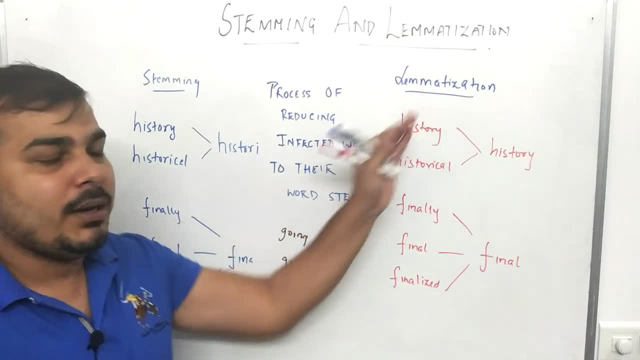 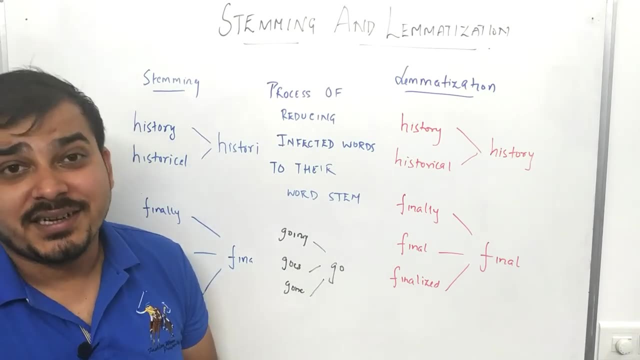 Okay Now why do we require stemming? Okay, We will come to limitization, but just understand why do we require stemming? Guys understand in NLP most of the use case that you have seen. there are use cases like sentiment analysis. 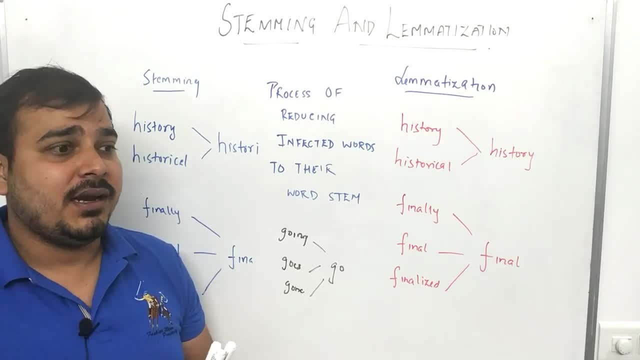 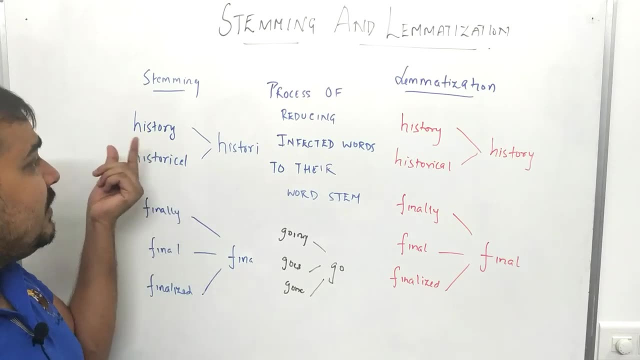 There are use case like determining spam classifier. There are use cases like to understand restaurant reviews and provide some ratings. You know, in that particular use case, the most important things in that particular words or the comments that people receive, People are actually putting, the most important things are basically the word, stem words. 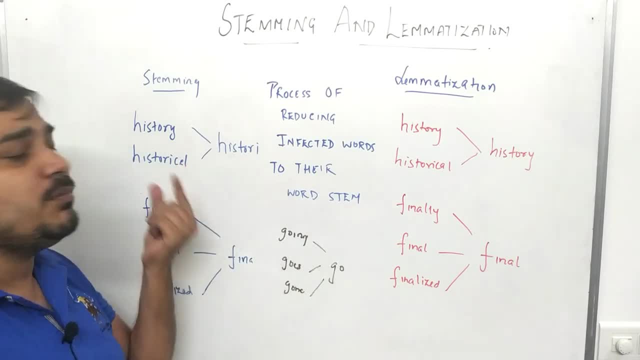 Okay, The stem, the word stem, which is the base word, right? That is pretty much important. by just having that particular word, we will be able to determine whether that word is positive or negative. Okay, So that is what is stemming. 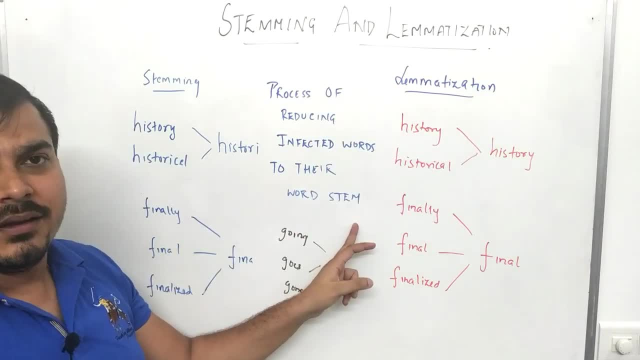 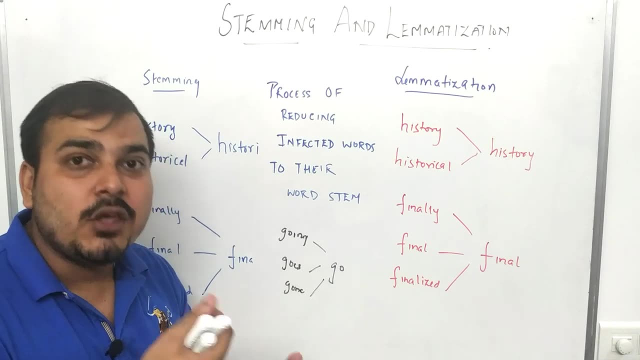 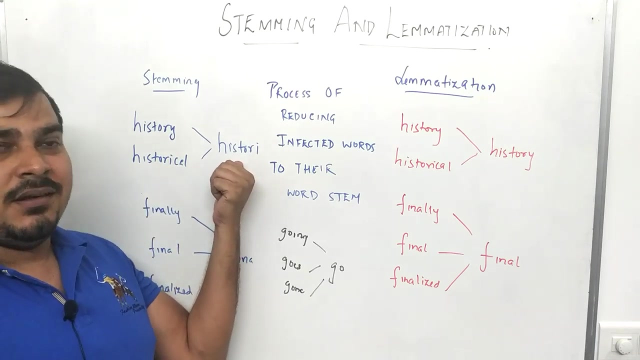 Now, what does limitization do? Limitization also does the same thing, but it converts that word and whatever word we are getting, it is a meaningful word, Basically understood by human being. You know it is a meaningful word In this particular situation. you can see history and historical get converted into history. H-I-S-T-U-R-I. 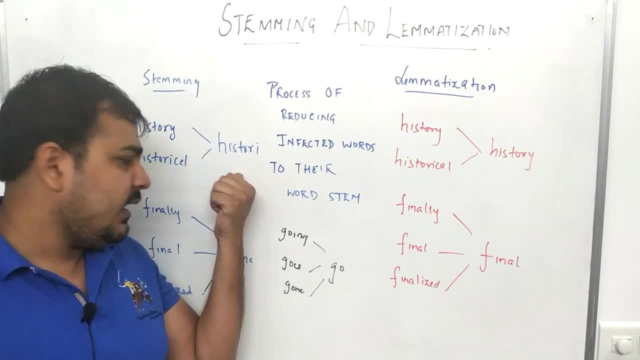 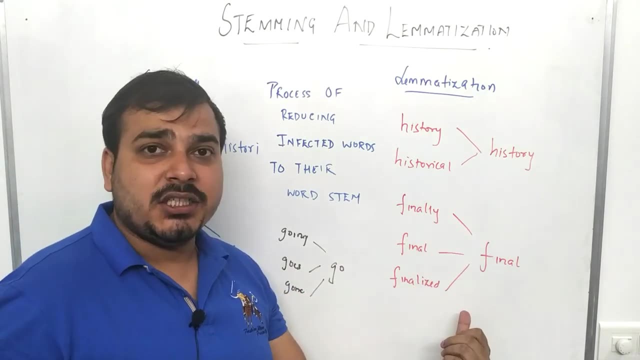 This will not make sense, right? What is this particular word all about, Right? Similarly, if I say finally, final and finalized, I'm getting fina F-I-N-A, But if I apply limitization here, I'm actually getting final. 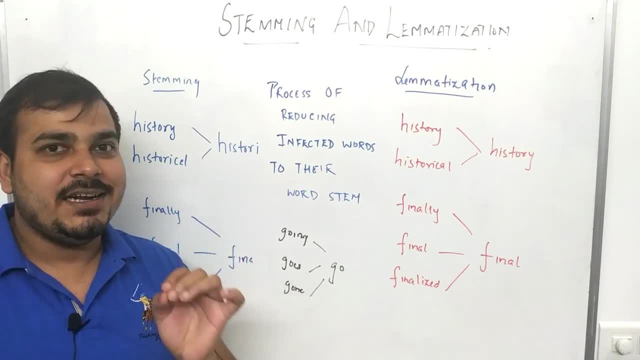 Right, And this all is possible by using a library which is called as NLTK, And in the future upcoming lessons, I'll also be coming with spaCy libraries, which is pretty much amazing. You know, spaCy library is also a very good library with respect to NLP work, that is, national language processing. 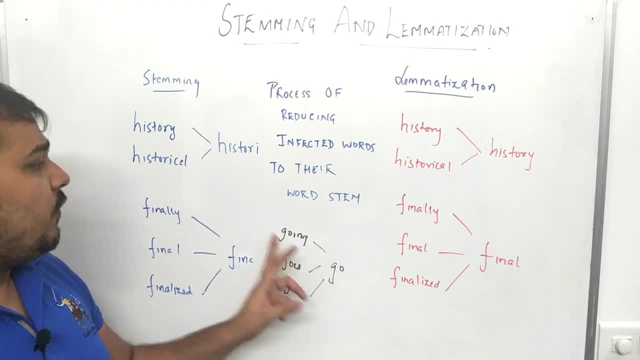 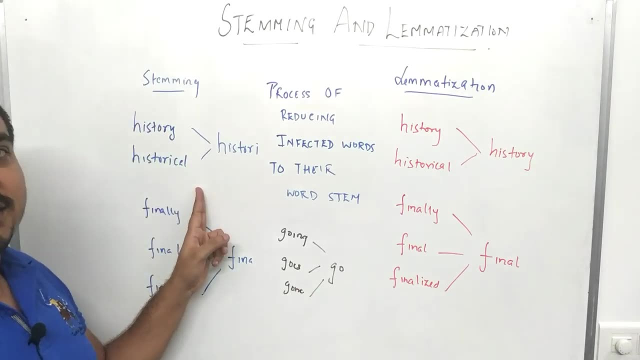 Right. But if I take this example of going, goes and gone, for all these three words, both stemming and limitization, also works, similar, You know. so for some of the words, stemming may not give you a proper representation, may not give you a meaningful representation. 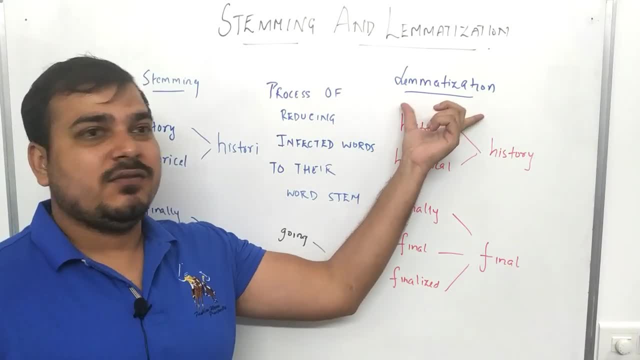 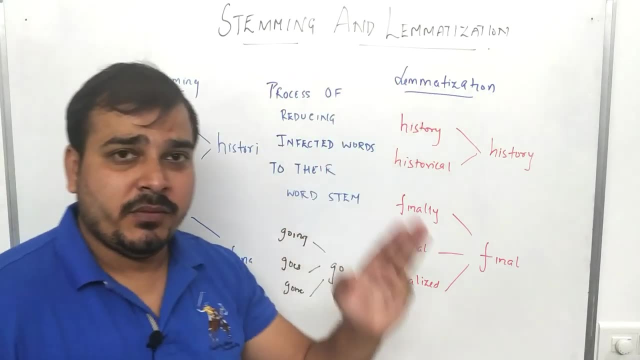 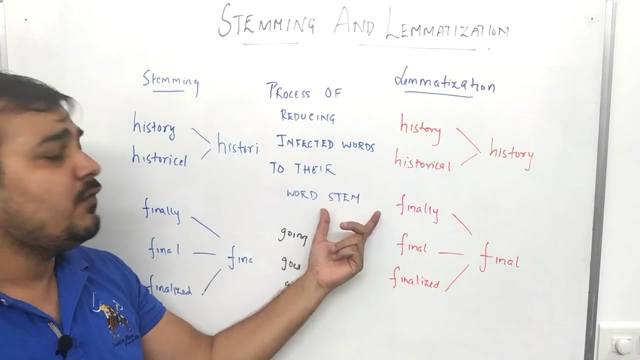 You know, the human being will not be able to understand, Whereas limitization is focused on giving a representation which is quite more meaningful. Now understand the basic difference Between stemming and limitization. The first you know difference is basically limitization. when it is converting or when it is giving another form of the word, it may it will definitely have some meaning. 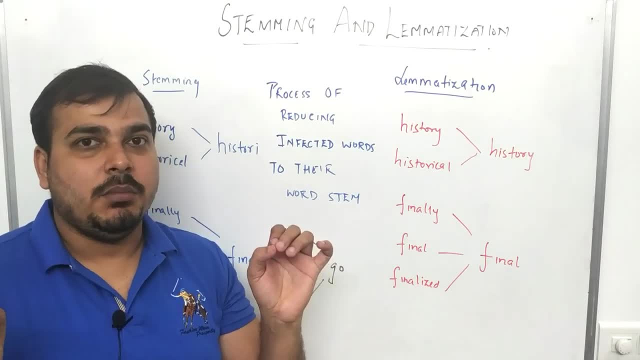 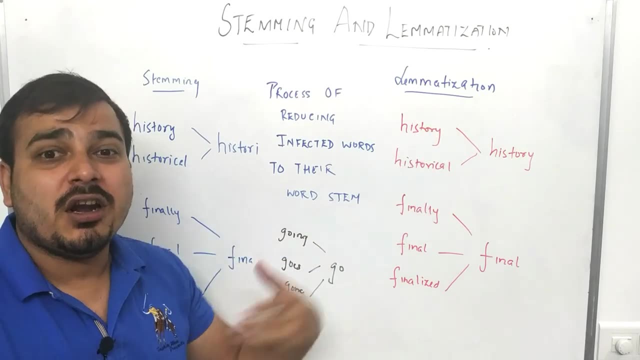 Whereas over here in stemming, the word representation will not have any meaning. You know, some of the word representation will not have any meaning. OK, The second difference is that limitization takes usually a lot of time, because to come to a meaningful word it usually takes time. 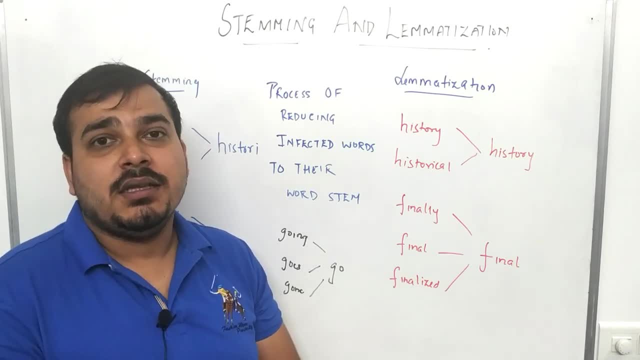 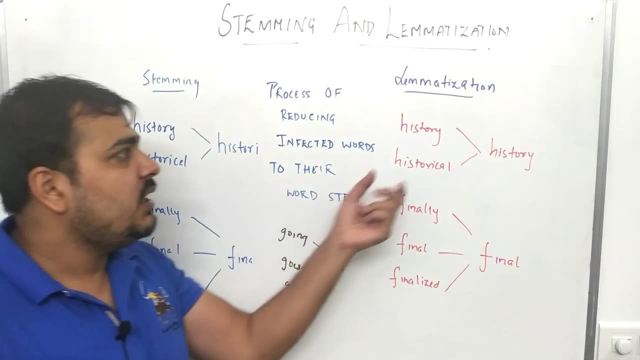 It has to do that processing, It needs to understand each and everything inside that particular word, Whereas in stemming it does not take that much time because it's just trying to find out the base word Right now. the third difference is that what all kind of applications we can use- limitization and stemming. 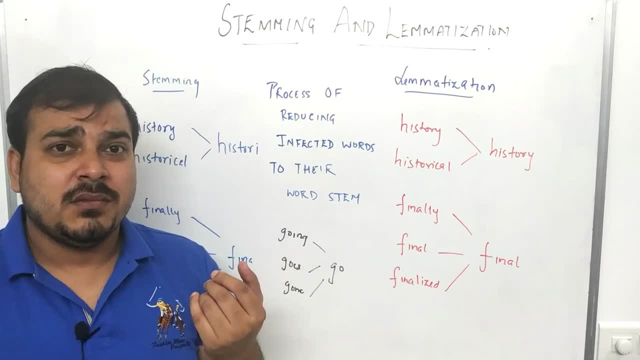 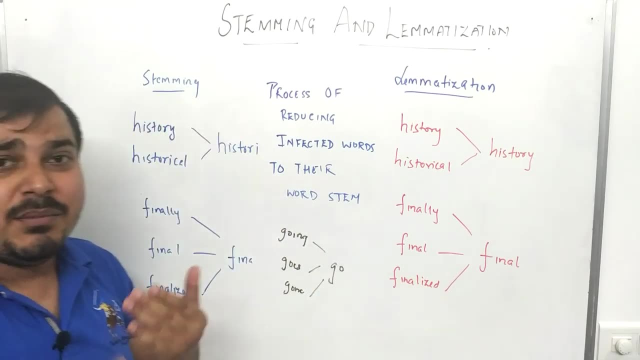 If I go to stemming guys, some of the application and sentiment classifier, you know. positive, negative sentiment analysis, Gmail classifier, you know. So these are, these are things can be used in stemming because, understand, we just need to find out the base word. 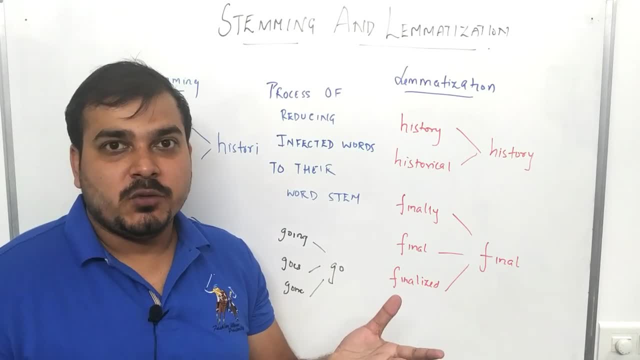 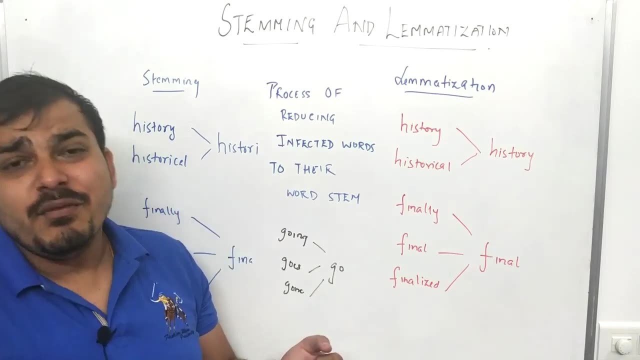 OK, we will not represent the word in the proper sentence. You know a proper meaning should not be there in the word. We're just trying to find out the base word. We have those data in our training data set and then we'll be able to determine the sentiment analysis. 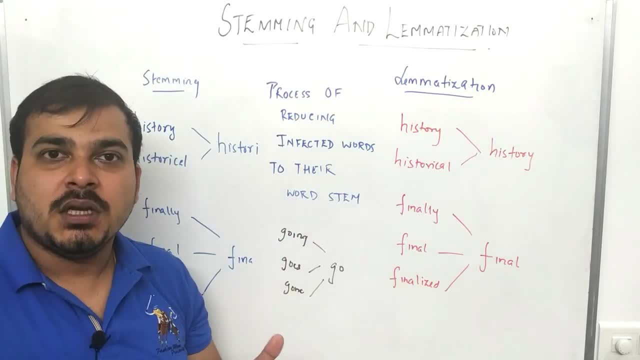 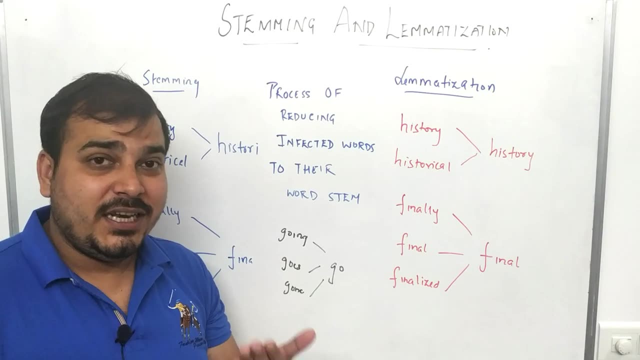 Whereas limitization used. limitization can be used in chatbots. It can be used in question answer application, because the response that a human gets from those application is meaningful Right. So we need to have that meaningful representation Right. So I hope you have understood about stemming and limitization. 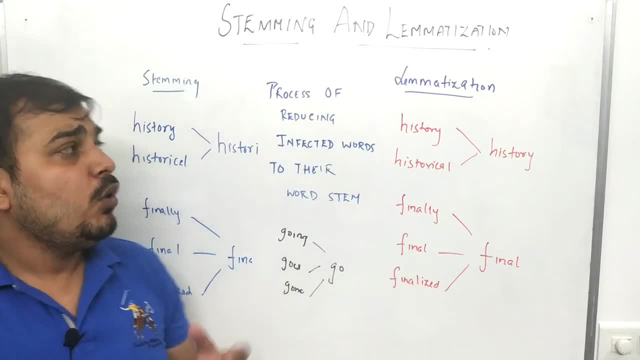 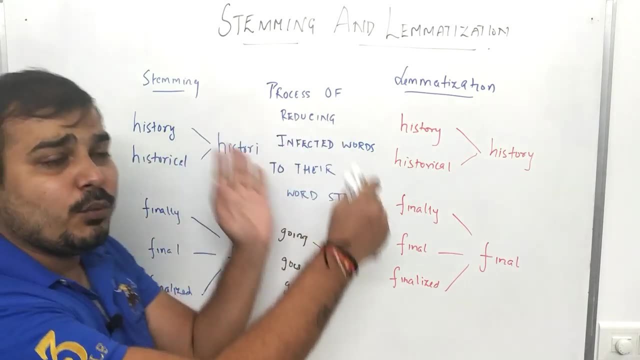 My next video will be with respect to bag of words: How we can actually implement bag of words. You know, with the help of NLTK library, that whole working. I'll be showing you how it works. I'll be taking a very good example. 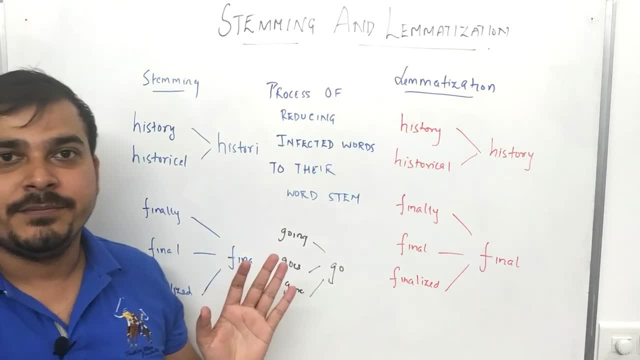 And what all things are computed in bag of words I'll be showing in this particular board itself. So yes, this is all about this particular video. I hope you like it. Please do subscribe the channel If you're not already subscribed. I'll see you in the next video. Have a great day. Thank you one and all, Bye, bye.